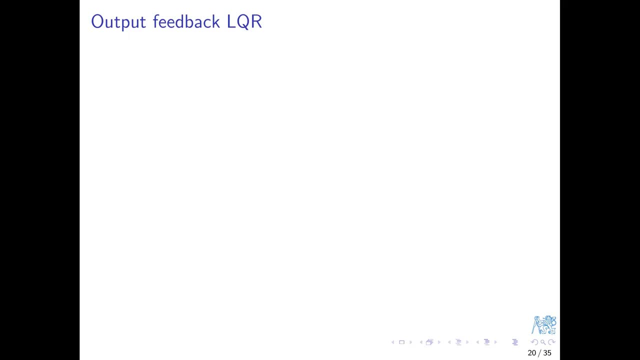 In this video, we will relax the assumption upon which we have been relying so far, namely the assumption that all the variables are measured and available for the feedback, Relaxation pretty much motivated by practical scenarios. This relaxation will be directly projected into our model. Besides, 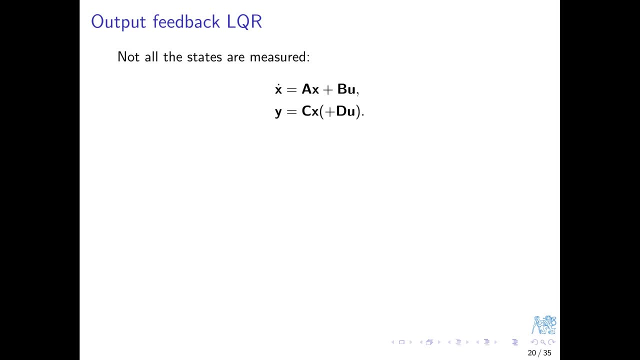 the standard state equation, we start using also the output equation. This is to say that instead of the state variables only some subset or possibly even some linear combination is measured. Know that very often in the introductory texts the D term- the direct feed-through- is assumed zero. 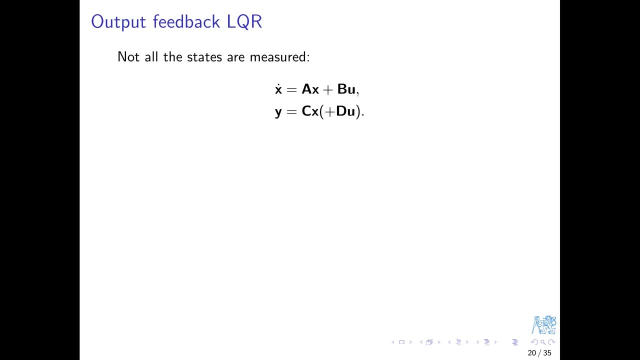 since some formulas are then a bit simpler, but here we do not particularly rely on it. The task is now to find a feedback controller K that takes the outputs Y and projects them directly into the controls U. It can be required to keep the controller just proportional, just an array of static gains. 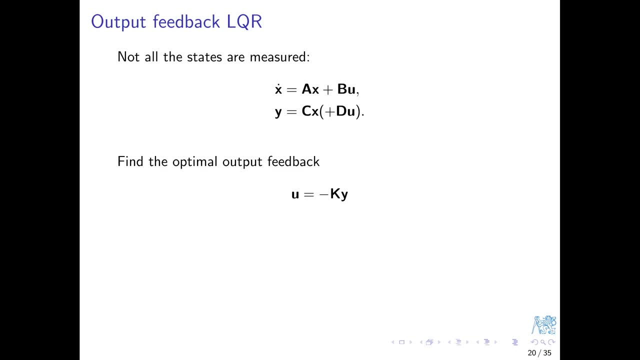 perhaps for the reasons of simplicity of implementation and commissioning, The controller should, as usual, stabilize the system and minimize the standard LQ cost. However practical this problem statement is, the trouble with it is that computationally it's surprisingly difficult. It's surprisingly difficult to design such controller As a 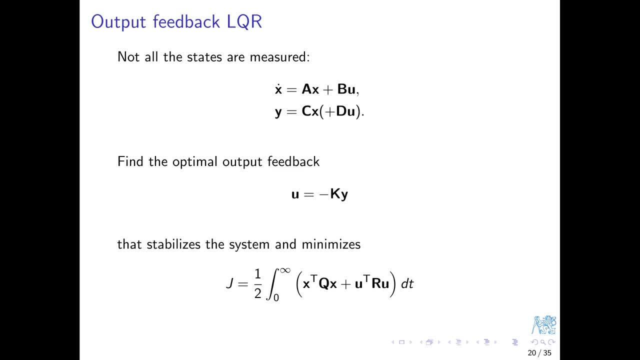 matter of fact, the difficulty does not come from the particular form of the cost function, but from the existence of requirements on the structure of the feedback controller. Indeed, once you fix the structure of the controller, be it a PID controller or, as in our case, just a matrix version of a 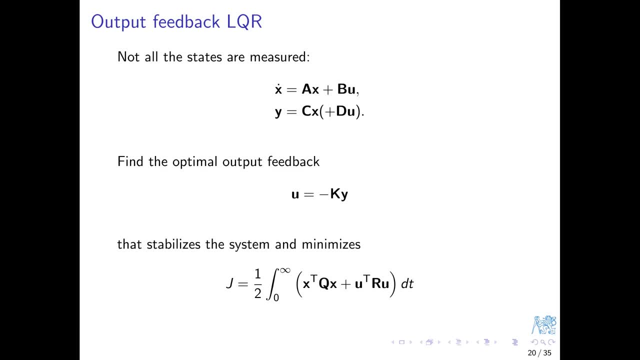 proportional controller, the computational task of finding stabilizing gains becomes non-convex, Hence computationally very challenging. Recall that previously- I mean in previous lectures- we did not require that LQ optimal controller be a state feedback controller. Instead, the form or the structure of the controller. 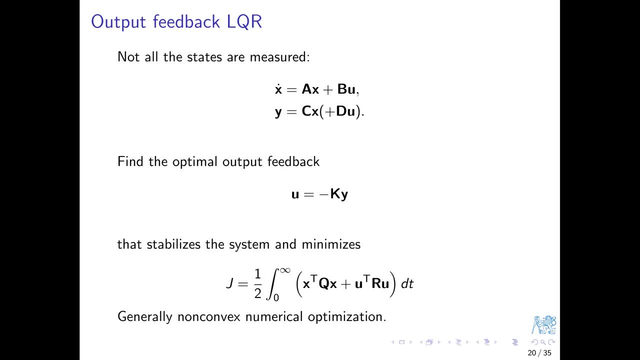 followed from the optimization. In contrast, here we are making an explicit constraint on the form of the controller. Well, in our course, I did not plan to go for this essentially research grade material, But should your project favor the LQ as a controller, then the LQ should be fine. 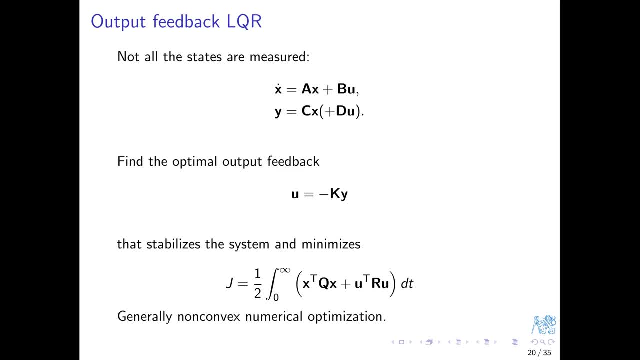 favors this problem formulation. I can at least inform you that various approaches exist. You may perhaps check Louis' book on optimal control, where a full chapter is dedicated to the problem, or search for constant output feedback keywords in IEEE Explore library. But my plan for now is to offer you 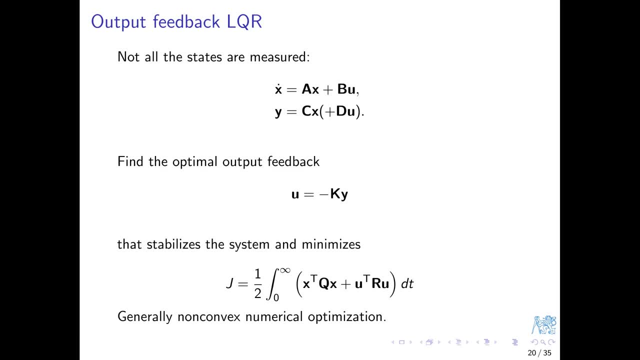 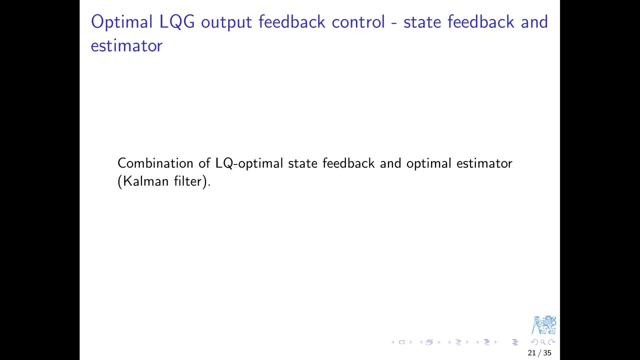 another framework, certainly a more mature one. The framework is well known under the label of LQG optimal control. It's based on a combination of an LQ optimal state feedback regulator and an optimal estimator, actually Kalman filter. We have had enough of the former in this course. Let's have a brief look into the 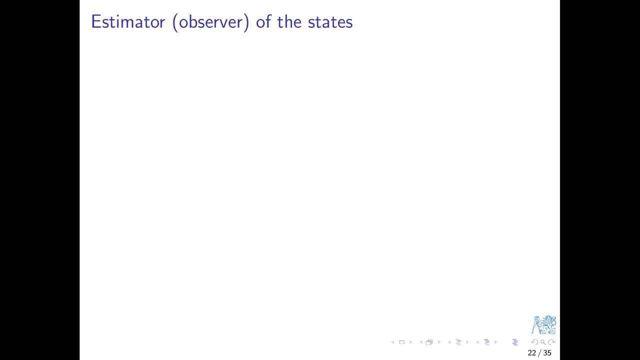 latter, It will also give us the clue. as for the letter G, G in the LQG abbreviation, We consider the standard LTI state space model given by the quadruple of matrices A, B, C and D. Here we assume D zero, for simplicity. 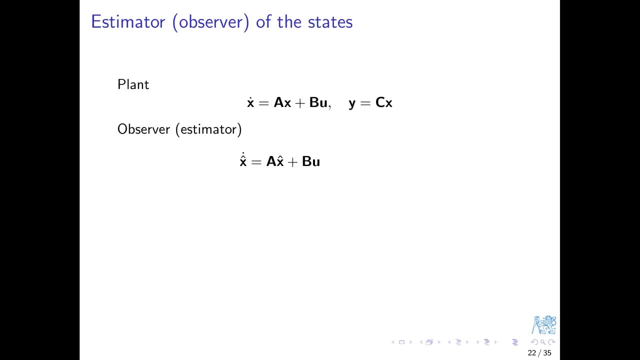 The observer or estimator is essentially model of the system, but this would not be enough, because the model is always just a model. Some correction must be introduced to make the observer practically usable. Putting related terms together: the structure of the observer, by the way. 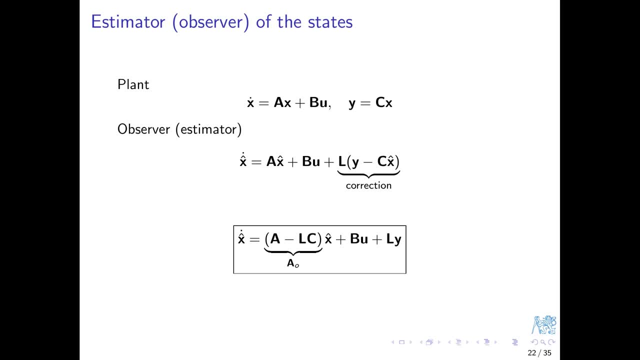 attributed to Lohenberger is more transparent. Its own dynamics is given by the closed-loop matrix A minus L times C, And there are two inputs to the observer: the input U to the system and the output U. The observer is parameterized through the matrix L of static gains. Now what is the 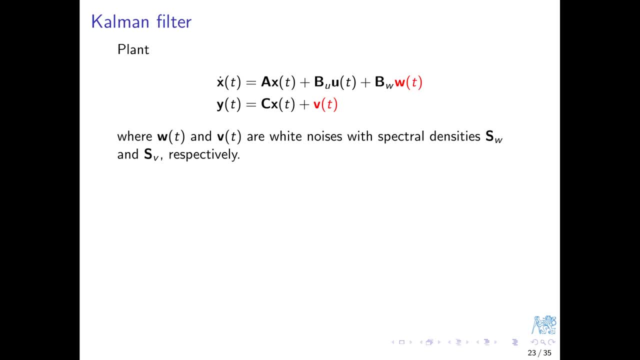 most typical relatively common filter. Let's start with linear equilibrium: CalCulTr, CalCulTr, CalCulTr. is항� bå Τ ans is1 n? Lg. Disturbance is what truly affects the system. 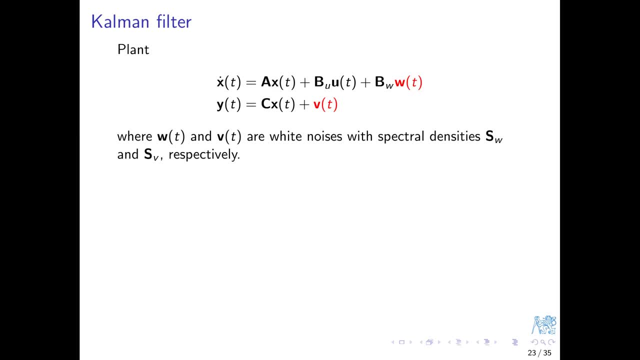 Noise or measurement. noise is what corrupts the measurements. Anyway, both are regarded as random variables. White noise with Gaussian normal distribution at a given time, with spectral densities SW and SV respectively. Now the origin of the letter G is clear. I guess G stands for Gaussian. 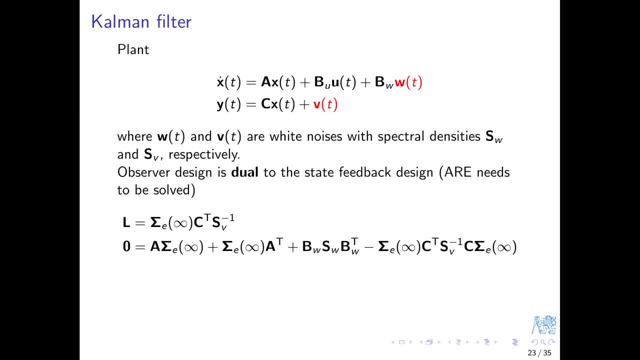 For this setup, the matrix L parameterizing the Lohenberger observer is desired, Postponing the theory to another course. let me just state that computationally, the task is dual to the LQ optimal state feedback problem. Suffice to say that this means that Riccati equation needs to be solved. 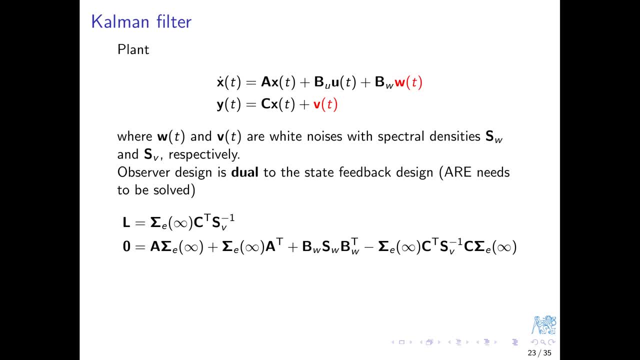 You will certainly be able to call the CARE solver in MATLAB with appropriate coefficients and then use the result to obtain the L coefficient for the observer. Note that the interpretation of the solution of the algebraic Riccati equation is that it is a covariance matrix of its estimation error. 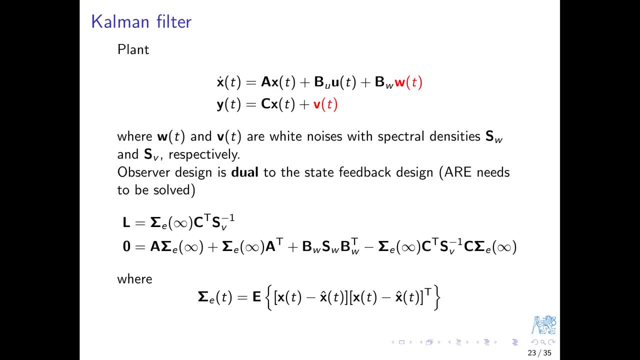 The optimal cost is then the trace of this covariance matrix, that is, the mean square value of the estimation. error. Theory aside, good news is that, again computationally, it is possible to solve this problem. Computational routines for this computation are available in perhaps any serious computational 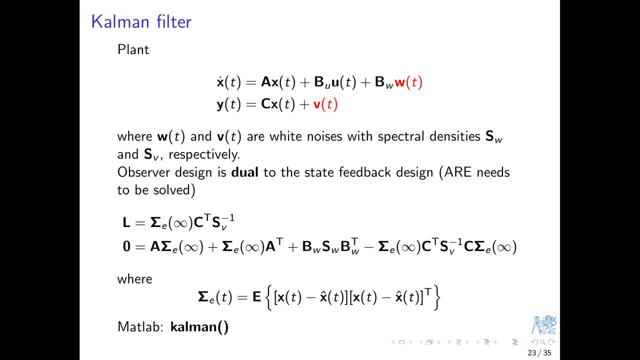 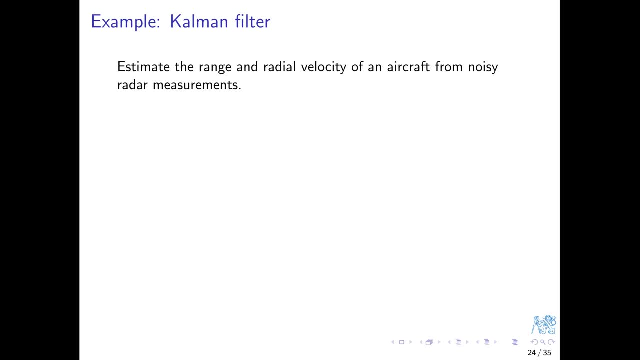 package In MATLAB. it is named, not surprisingly, Kalman. Simple example on Kalman filter: Estimate the range and radial velocity of an aircraft from noisy radar measurements of its position only. The model is just a double integrator. The state variables are the range or distance r and its derivative, the radial velocity. 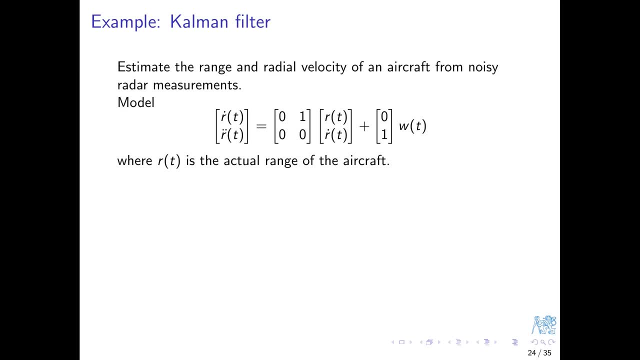 not that? the very problem of estimation has nothing to do with control and therefore in the model we do not even need to model how the control signal enters. Instead, we do have to specify or model how the disturbance torque affects the system. 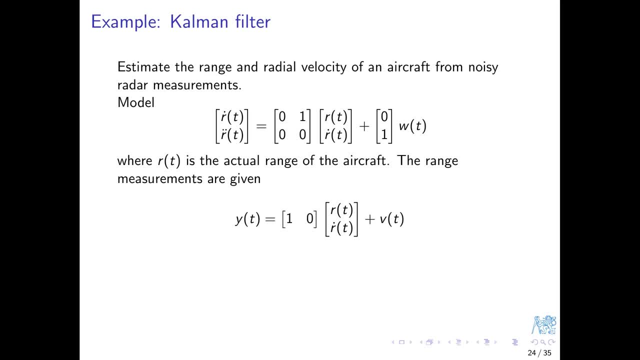 We also need to specify the output equation. It tells us that it is only one of the two state variables that is measured. This is This I have already mentioned- and it's only the range that is measured. And the equation also shows that the measurement noise is directly added to the measurement. 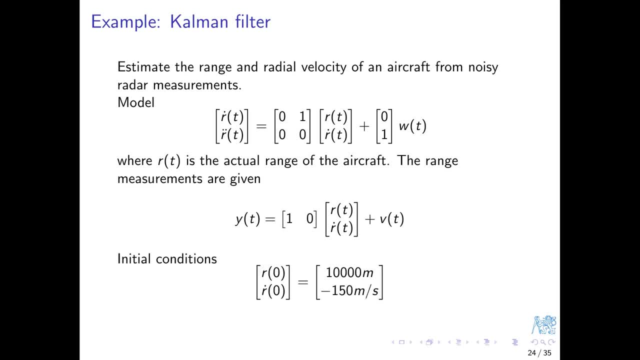 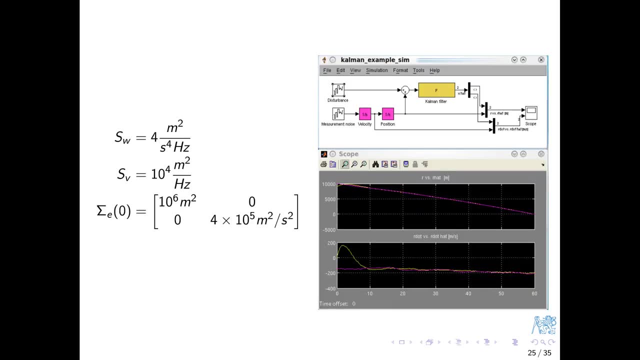 of the position. It's an additive noise. Initial position and initial velocity are specified. The implementation of both the design procedure and the simulation in Simulink can be downloaded on the course website. You can see that the initial, The initial discrepancy between the estimated and true states diminishes. 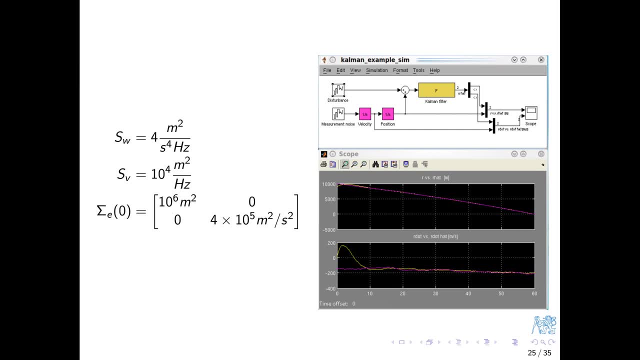 But the system is exposed to random disturbances and therefore the estimation error never really decays perfectly. it never really goes to zero exactly, But the mathematics behind the design guarantees that it is as small as possible in the mean square sense, and under those special conditions. these we should keep in mind. Gaussian white. 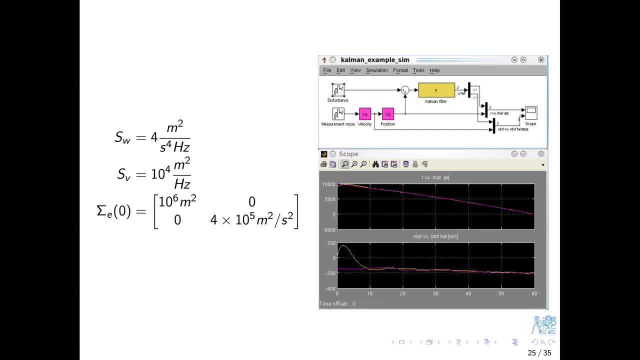 noise as models for both disturbance and measurement noise. Moreover, these two should be independent. Practically speaking, determining the spectral densities SW and SV can be difficult, but without diminishing the value of those attempts to estimate these parameters, I can propose an engineering attitude. 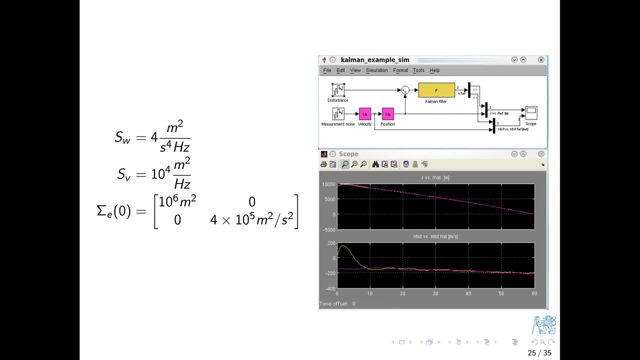 The two coefficients or coefficient matrices play the same role in the computation that the Q and R matrices played in the LQR design. Therefore they can be viewed as sort of kind of tuning knobs. Again, it's not their absolute values but rather ratios between the two that matters. 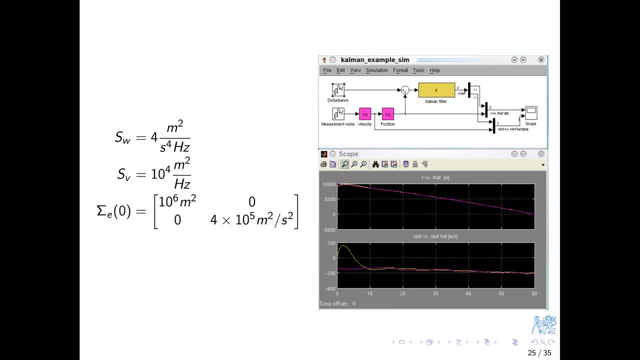 Setting the coefficients in the SW matrix higher than those in SV means that we expect more intensive disturbance, and therefore we should trust the model less than we trust the measurements. If it's the other way around and the coefficients in SV are higher, this reflects the fact that 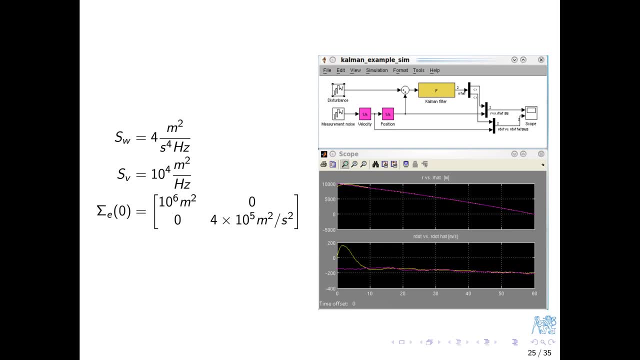 we expect more intensive disturbance And therefore we should trust the model less than we trust the measurements. This reflects the fact that we anticipate heavy measurement noise. that makes the measurement less trustworthy and we rely more on the model. If you have not been exposed to the design of Kalman filter yet, try a few iterations. 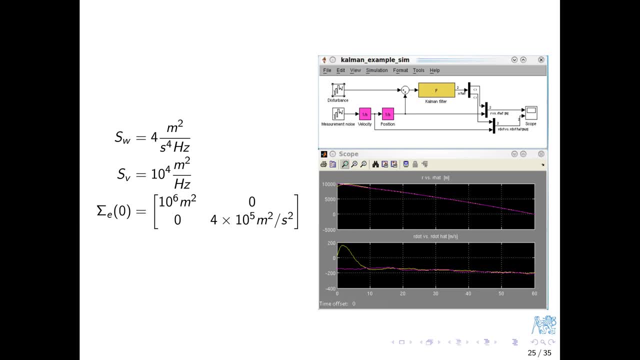 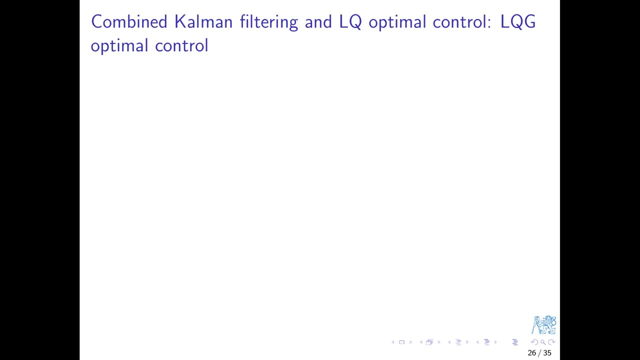 by yourself with the provided models and code. Good, Now combine the two, the LQR state feedback and the Kalman filter, to form an output LQG controller. The way to combine the two, in fact, the general state feedback and the general observer, not. 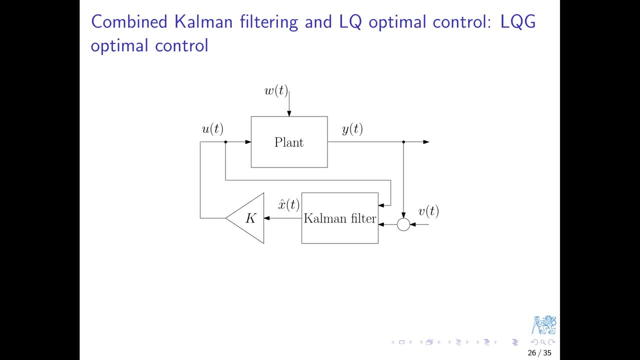 just the optimal ones is in the block diagram, a reminder. computationally, the design amounts to solving two algebraic Riccati equations, one for the optimal state feedback and one for the Kalman filter. But in MATLAB you can use just those. 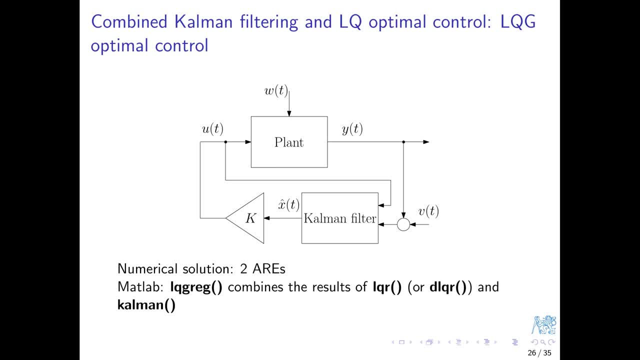 Just those. Then convenient higher-level design routines: LQR or DLQR in the discrete-time setting for the LQR state feedback and Kalman for Kalman filter design, And then LQG reg to glue it all together. Example: 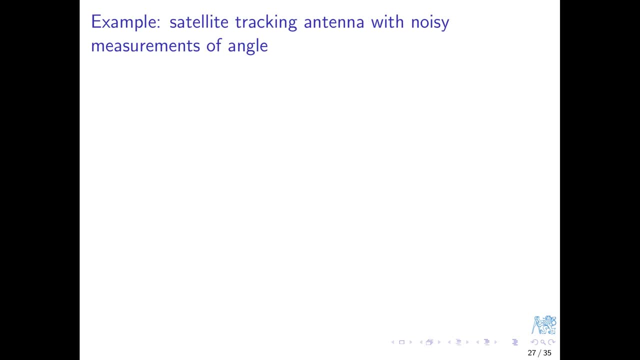 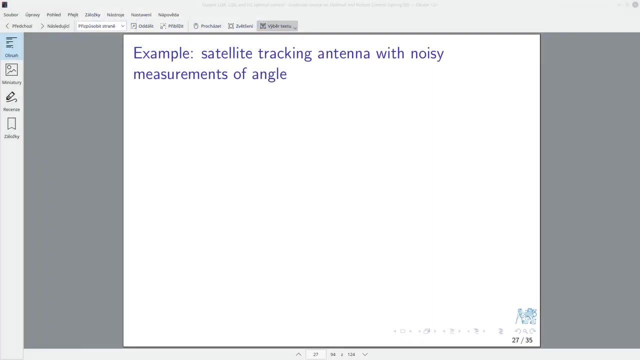 Here we combine the previous two examples on Stochastic LQR and Kalman filter. You know what? I will finally launch my own MATLAB and play a bit with the design and the simulation. so let's get out of the presentation and let me show you what. 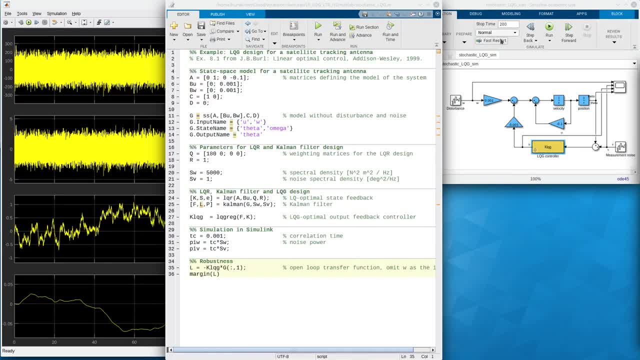 I've prepared. so here comes the code. then I have the Simulink model for the simulation and of course the scope with the simulations from some previous run. but let's first start with the the code here. so in the first block you can see that I built the matrices defining the state space model and to note that I 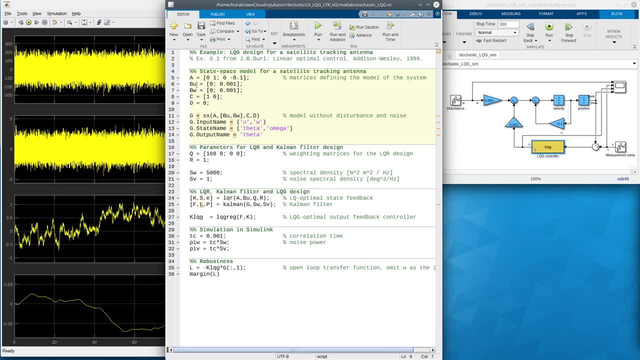 have the two B matrices here, one corresponding to the control input- you- and the other corresponding to the disturbance. then I built the state space model. for convenience I also labeled the information here and then I saved it like that: inputs, the states and the outputs. but what then matters from the computational point of view is: 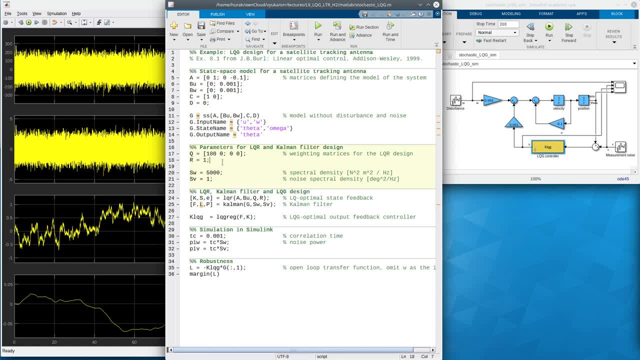 these parameters. here these are. this is actually the the place in the whole code where i, as an engineer, design something or or make some decisions so i can set the penalty on the states and the controls. we can see that here. the initial setting is that i only penalize the first of the two. 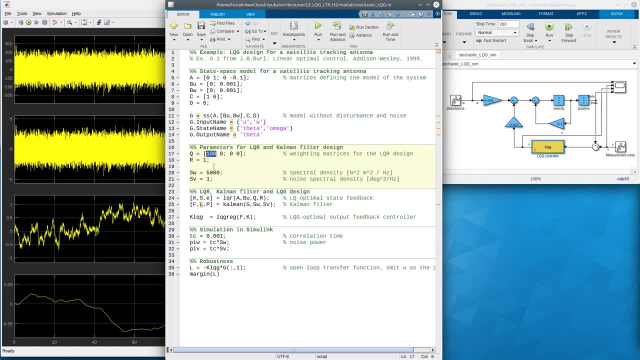 states. i only penalize the, the distance and not the velocity. i don't care about the velocity. and then i have the two guesses at spectral densities for the two random variables, sw for the disturbance and sv for the measurement noise. then in this block i'm designing state feedback. 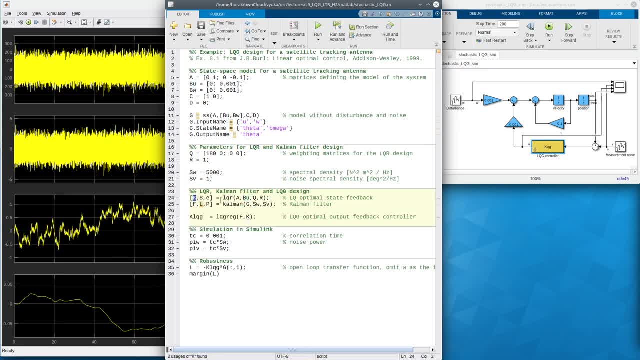 the result is then stored in the k variable and kalman filter, the matrix or vector of coefficients that parameterizes this observer. kalman filter is l, and then, as i've already mentioned, there is this convenience function, lqg reg, that puts it all together to form just a dynamic output feedback control. dynamic, i mean. 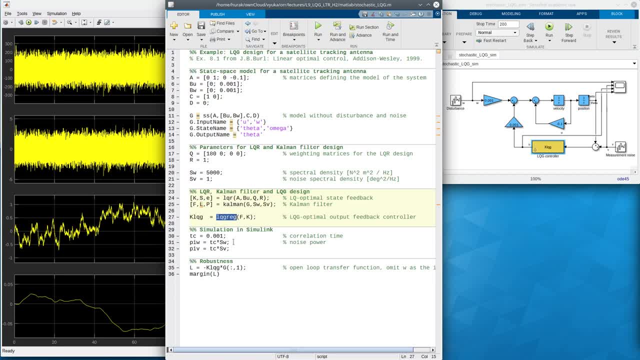 higher order, not just a static one. then in this somewhat technical block in which i'm translating the information that i have about the random variables, here the, in particular the spectral density, i translate it here into, or or transform it here into some other coefficients expected by by the simulink random random signal blocks. you. 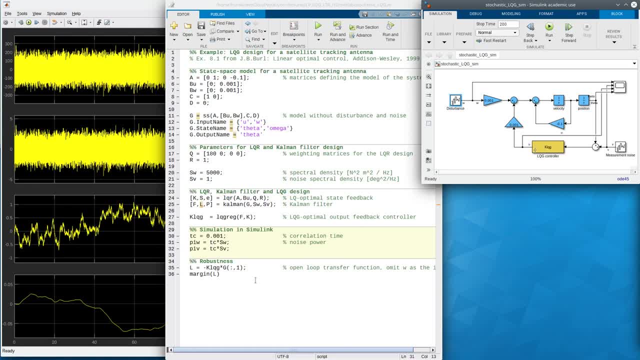 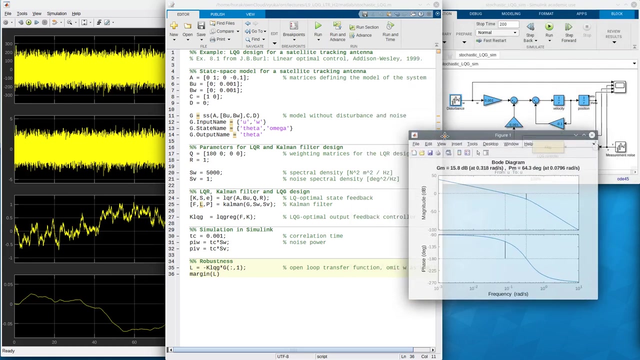 will find the details in the in the user's manual. and for out of curiosity or or in addition to the design, i can also plot or analyze, analyze stability margins here. so let's go for it. i will run design. you see that here is the open loop transfer function with the. 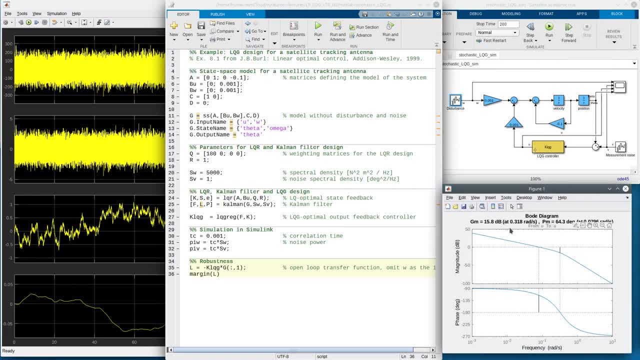 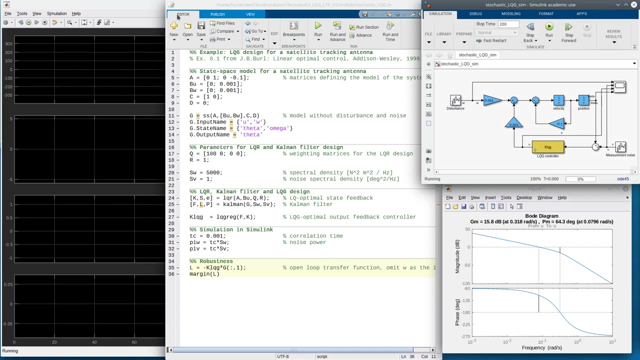 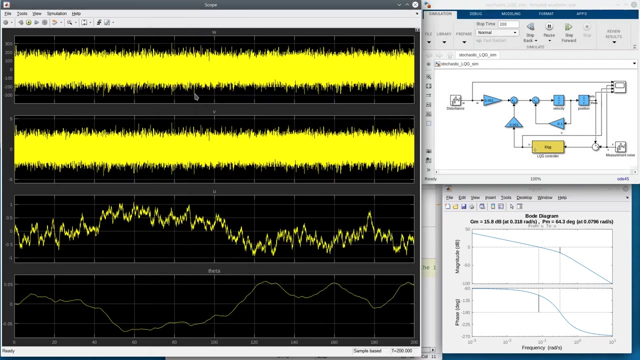 gain and phase margins already computed. so already this seems quite, quite nice. some 60 degrees phase margin and 15 decibel gain margin- pretty decent. let's now run the simulation. essentially i get what i had there before, but now let's have a look at these outcomes. so the first 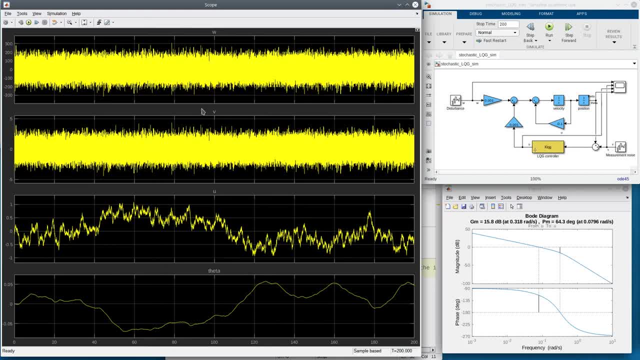 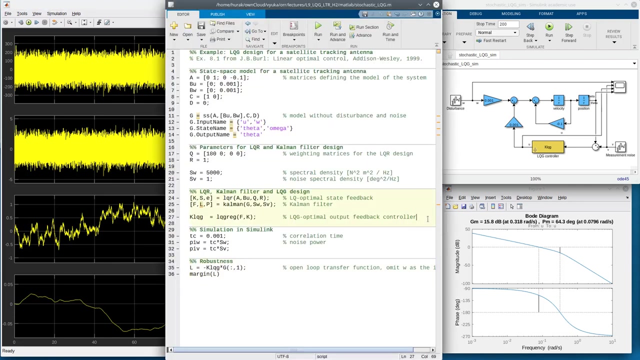 two signals. the random signals are the disturbance and the measurement. so the first one is for the and for this over here. and plus 0.05 say we are not quite happy about it. we want to make this regulation error smaller. so what's, what shall we do about it? we can penalize the. 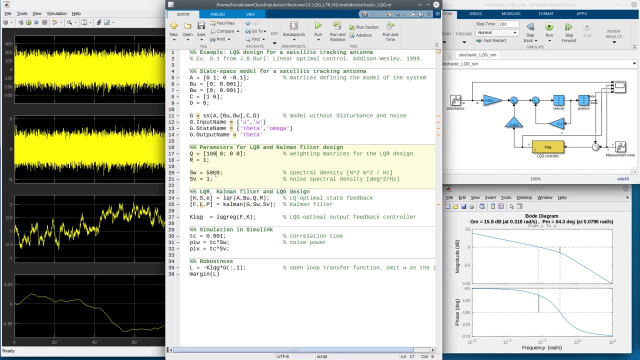 corresponding state variable. we can in by increasing the, the corresponding element in the Q matrix. say: increase it hundred times. remember this is quadratic. all right, so let's rerun the design. if you are not familiar with, or not that much familiar with, MATLAB, then note that this K? LQG is really some. 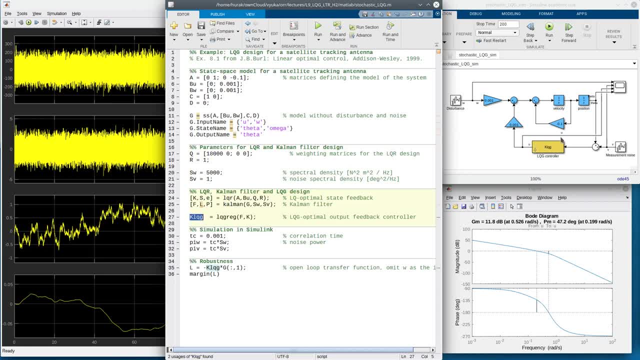 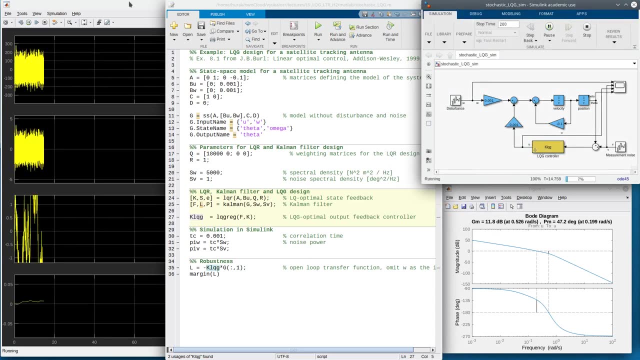 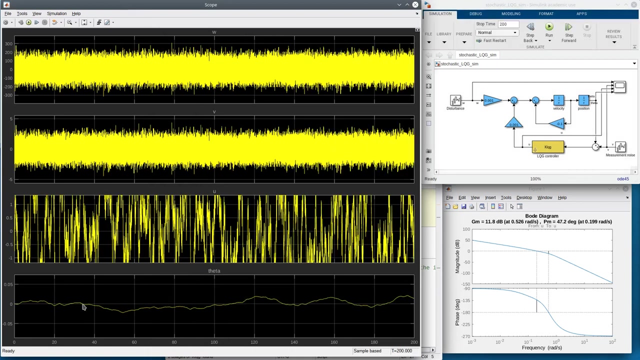 object. then here within a Simulink, I'm just entering the the name of this object. so this is this is how I get the results from MATLAB into Simulink. now let's run the simulation and see what happens. obviously I achieved what I wanted. the regulation error now seems reduced quite 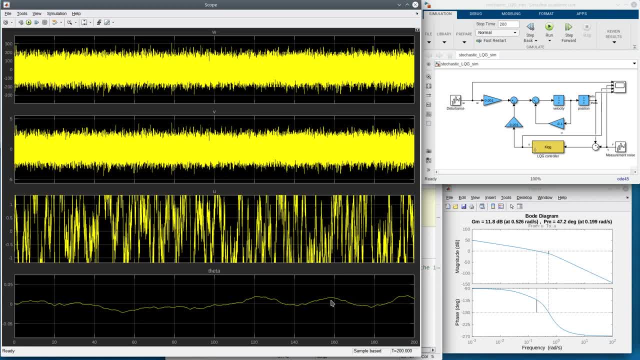 significantly, but of course this comes. this regulation error is now reduced quite significantly, but of course this comes. this regulation error now seems reduced quite significantly, but of course this comes. this reduction comes at a cost, and the cost is clearly that the control signal is, and the cost is clearly that the control signal is larger. right, and that's it. yeah, you may also. 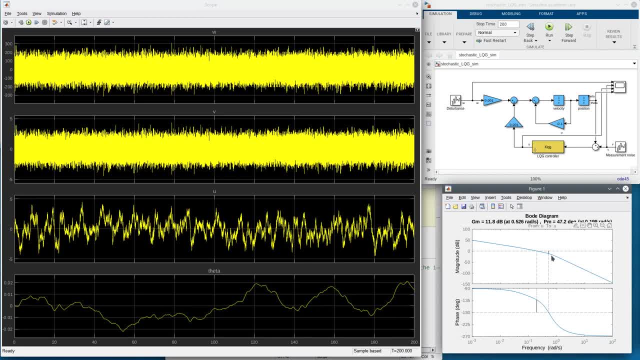 notice that by requiring more, a little bit more aggressive controller, the face margin is decreased, the gain margin as well, but still quite acceptable. all right, I think that's. that was enough for the illustration, and it's now up to you, if you, if you want to play with it a little. 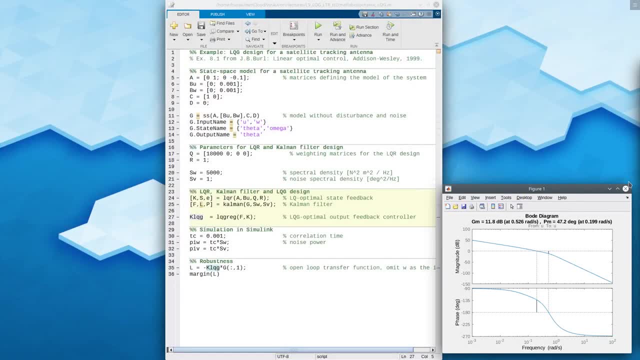 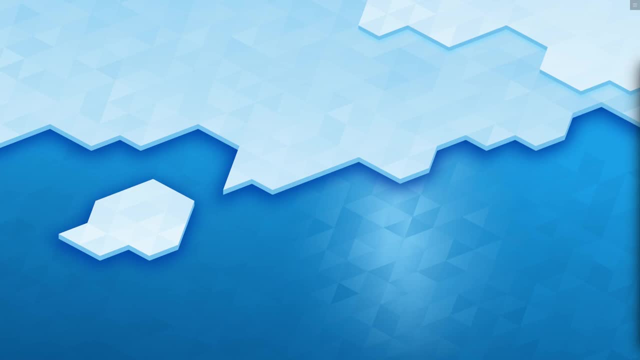 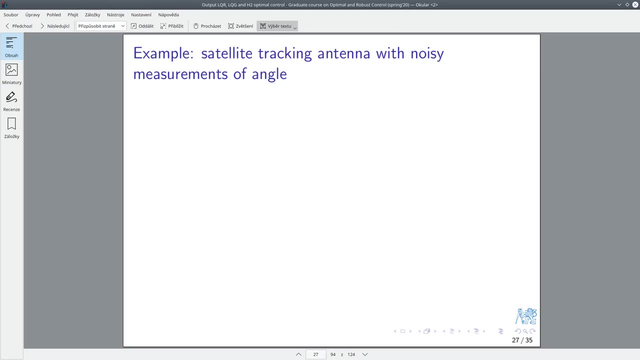 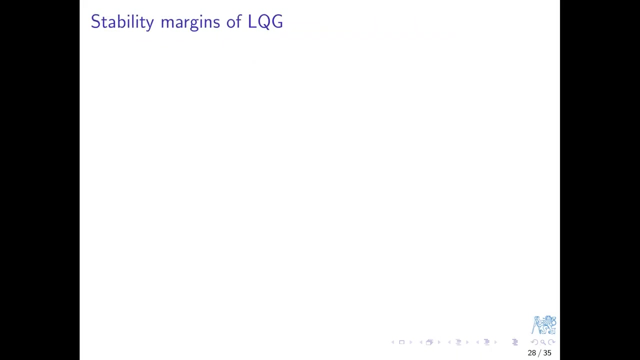 little bit more, So let's close it This one as well. Where's now the presentation Right here, So let's move on Right. we have seen some basic usage of computational tools for design of LQG, optimal output feedback controller or regulator. actually, The impression so far was great. I hope so. 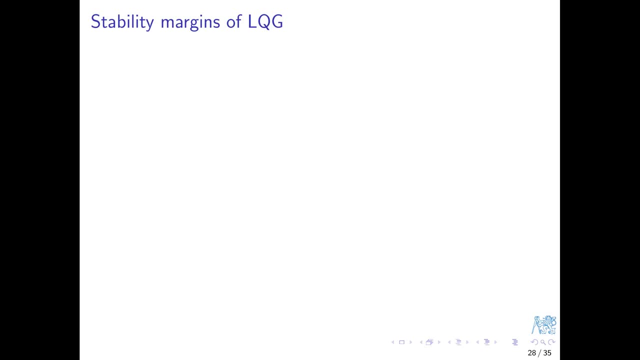 Just four types of tuning knobs- Q and R and SW and SV- with which we conveniently search for the right trade-off between aggressiveness and economy of control and reliance on model and reliance on the measurements. But life's not easy, is it? Let's have a look at stability margins a little bit. 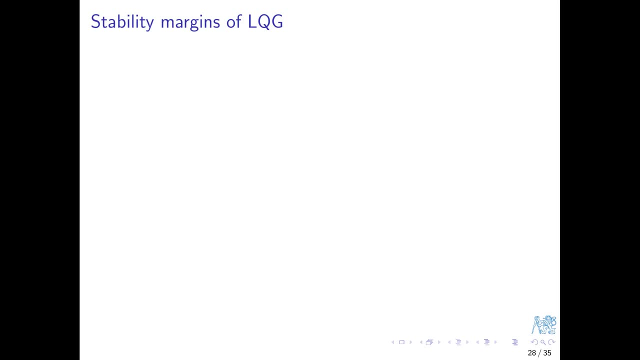 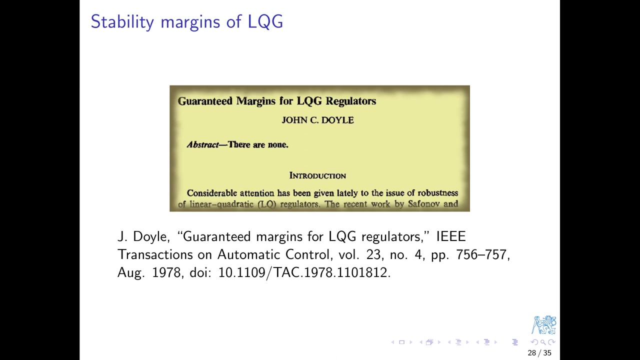 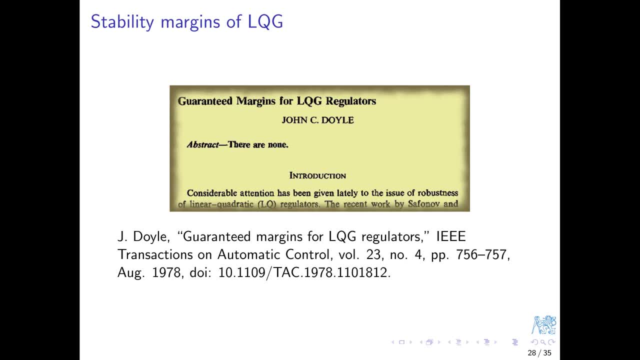 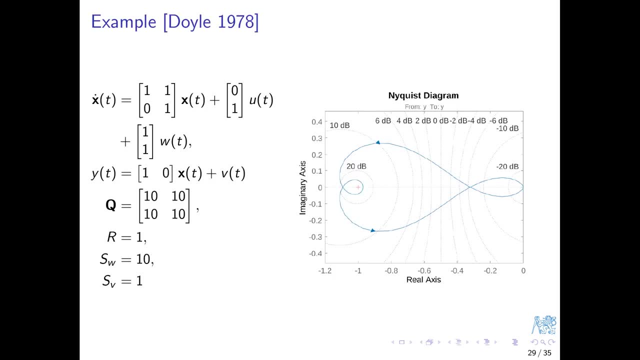 This was perhaps the shortest abstract of a scientific paper that I've ever read. In fact, the whole paper revolves around a counterexample. Here it goes For the system. for the given system, you can find the values of Q, R, SW and SV. 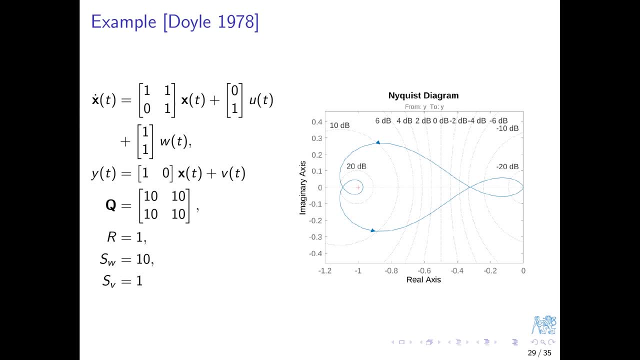 parameters such that the stability margin, stability margins, are arbitrarily small. Bad luck. In fact, this observation that was made back in the 70s started a quest for some other design techniques. Well, the frustration, some sort of frustration was already felt by the 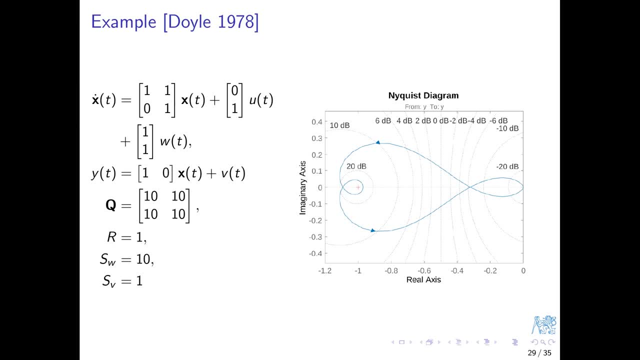 engineering community in those days because those LQG techniques. they did really a good job in the space domain, in which the were pretty accurate, but then they failed miserably when engineers try to apply them in some more down-to-earth engineering applications because of 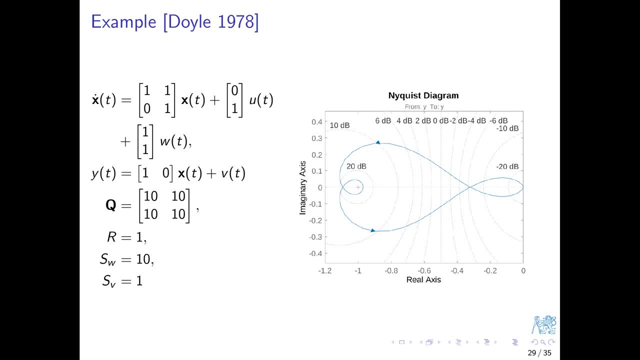 their lack of accurate models and lack of robustness of the LQG, as John Doyle formally proved. In the rest of the course we will essentially explore what are various alternatives, what are the options or more robust methods, And we start right away. We introduce a heuristic modification of 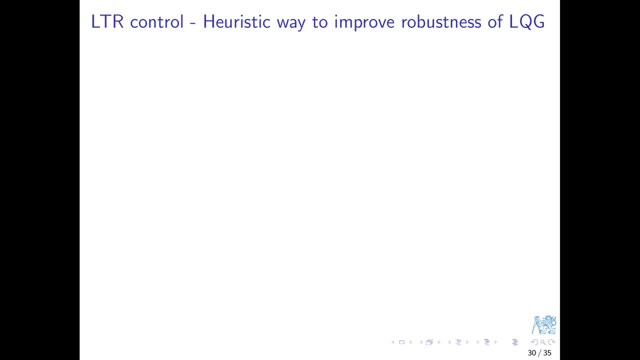 the LQG design procedure that aims at improving the robustness. The technique is called loop transfer recovery or just simply LTR control. The key idea is make the LQG a bit similar to LQR, That is, make the Kalman filter rely a little bit less on. 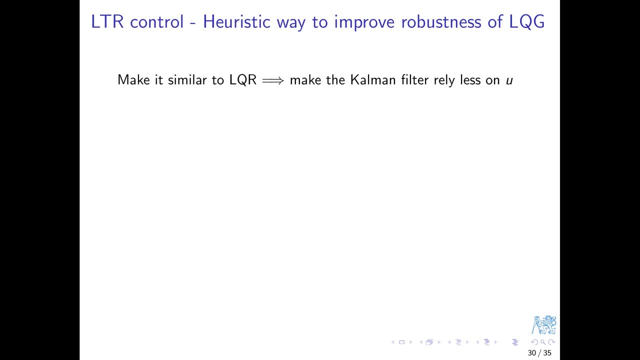 the knowledge of you. You will see what I mean right away. Kalman filter receives the input to the system as one of its two inputs. right, But the trouble is that there's typically some unmodeled dynamics around the input to the system which demonstrates itself as if the input was. 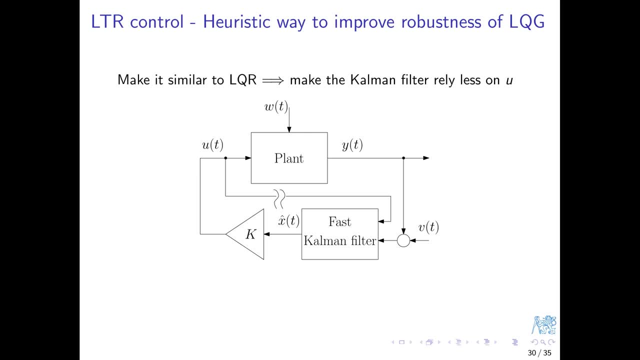 actually rather different than what the controller sends there. In this sense, Kalman filter is being fooled because it receives an incorrect information. Therefore, a good idea is to cancel, or at least weaken, the signal path from the control input to the system, actually the computed control signal, the signal. 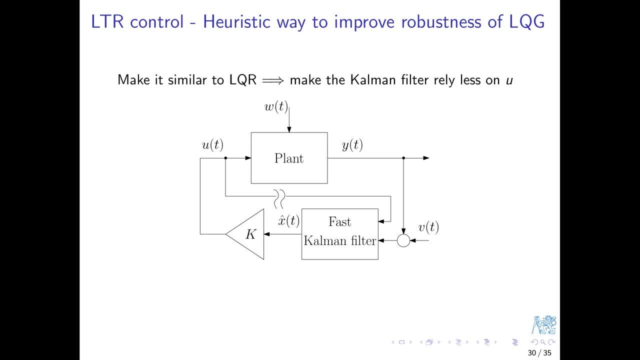 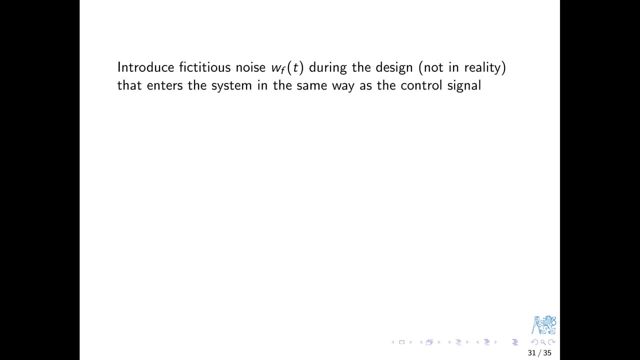 produced by the controller to the Kalman filter input. But how can we do that? The idea is this: Simply introduce some fictitious noise WF. I mean introduce it only in the design phase. I do not certainly suggest introducing whatever physical noise to the real system And this noise 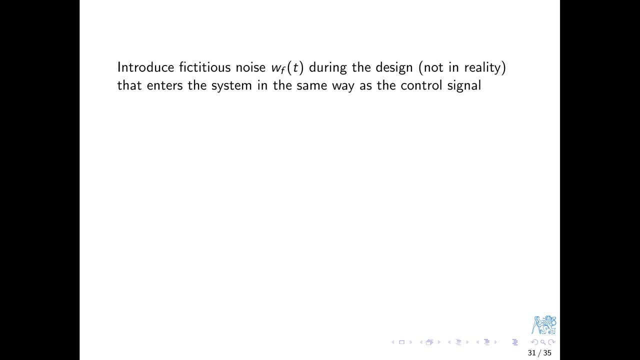 should enter the system or the model in the same way the control signal does. This is how the state equation changes. then For the new noise we also have to provide the spectral density SWF. but since the noise is really just a computational construct, it's artificial. the 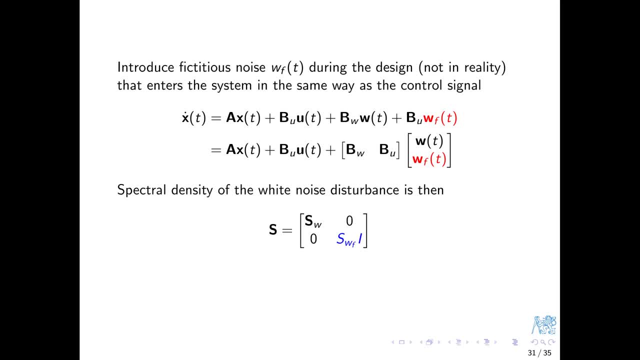 corresponding spectral density is nothing but a tuning knob for us. It has no physical meaning But increasing its value. we are fooling the LQG design procedure to think that the input to the system is horribly affected by some disturbance and that common filter should incorporate this. 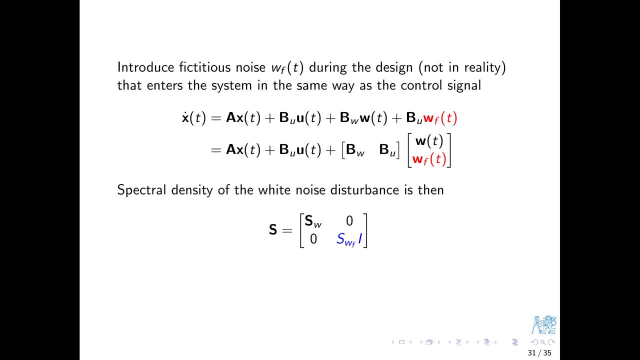 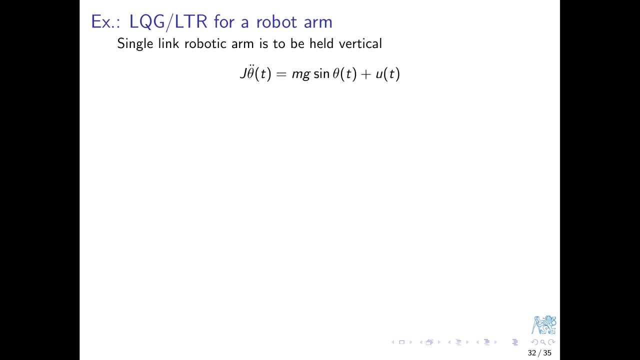 somehow, And that's it. You will find some quite elaborate theoretical treatments in the literature, but the core idea is essentially this simple and intuitive. Let's have a look at an example: A model of a single-link robotic arm. Linearized state equation is this: where W is a disturbing torque with a given spectral. 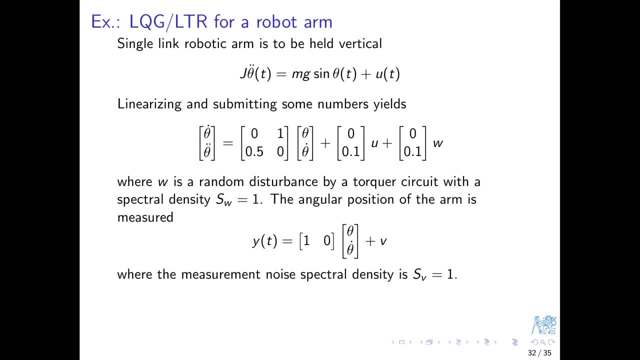 density SW and the output equation shows that it's only the angle of the arm that's measured and that the measurement is corrupted by the noise V of a given spectral density SV. The cost to be minimized is the standard combined mean square value of LQG design procedure. 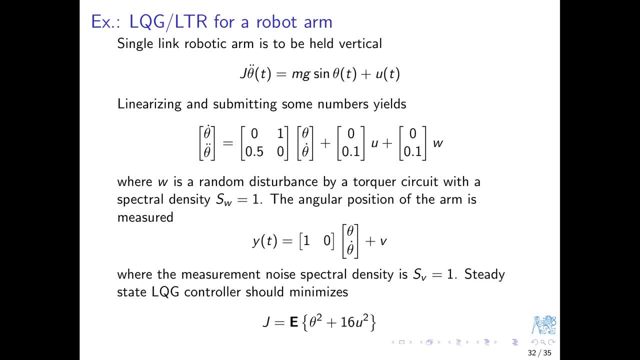 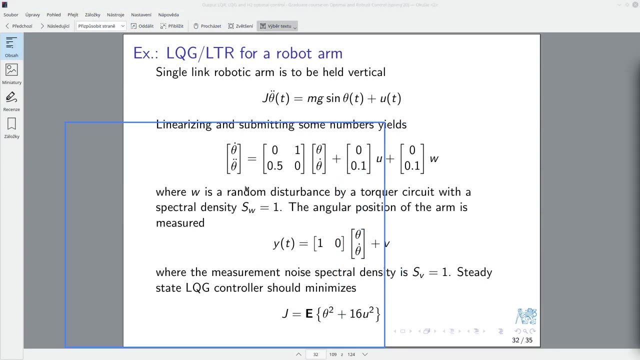 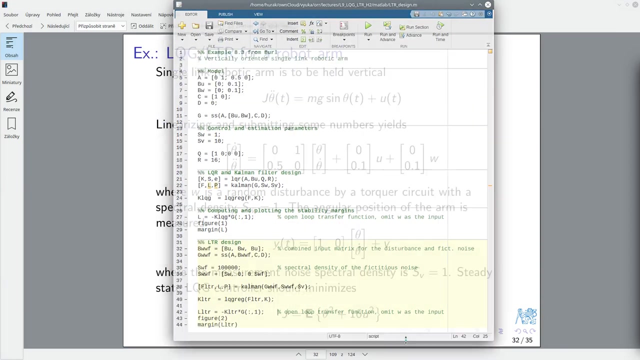 In this example the speed of the angular regulation error and the control. let me now comment a little bit on the design and the results in MATLAB again. so let's do it this way. So here comes the design code. Let me first go through it swiftly. 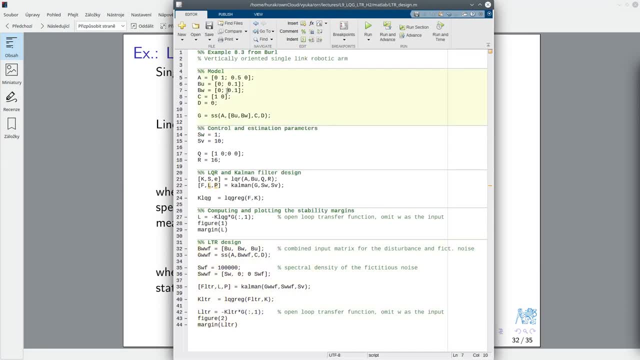 and only then discuss the憗s function very briefly, and only then discuss the憗s function very briefly. then I will run it So again, as we had before: state-space matrices, again splitting the B matrix into two parts, one corresponding to the controller, the 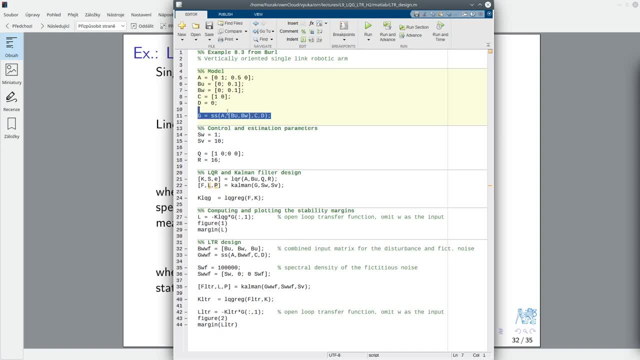 other corresponding to the disturbance. then building the state-space model, setting the spectral densities for the disturbance and the noise, setting the weighting matrices for the LQR stuff, designing the LQR, designing Kalman, combining them, computing the open loop transfer. 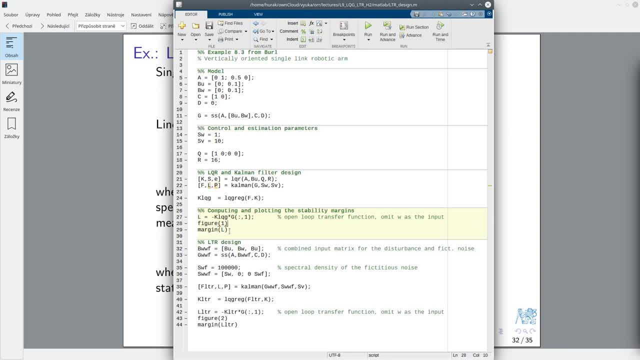 function and plotting it and computing the margins. So that's again. I forgot to emphasize it. this initial part of the code is just the sort of solver base standard LQR, just as a reference here, and here comes actually the the LTR design. so the only 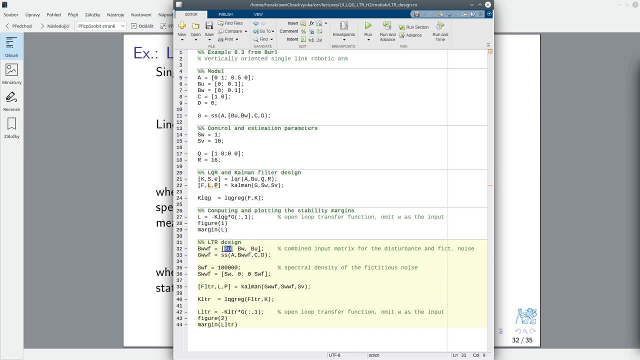 thing that we do is that we extend our original B matrix formed by these two matrices. we extend it with a new B matrix, but this one is identical to the B corresponding to the control right. so this is our new B matrix and with this new B matrix we build a new auxiliary or extended. 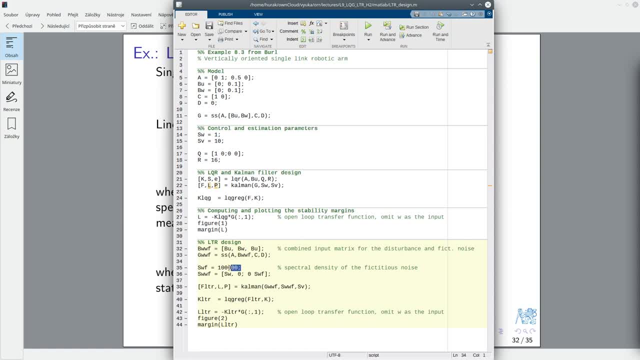 auxiliary system. then we set the spectral density for our artificial noise and we set it somehow unrealistically, or I mean arbitrarily high, just really to fool the system to think that I mean the control system, to think that the system is not real and that the control system is not real and that the control system 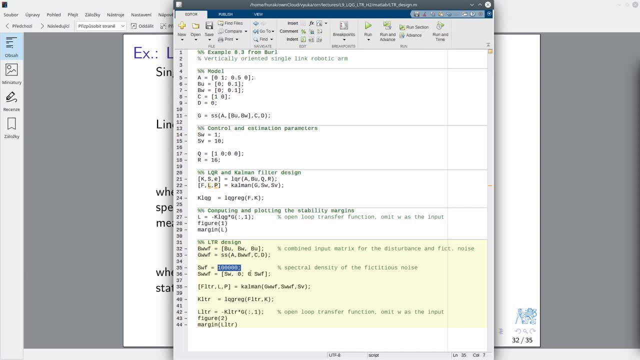 is heavily loaded by the disturbance at the input. then we form spectral density matrix for the augmented system and design a new Kalman filter. you see, we leave the optimal state feedback intact. we are only changing or designing new Kalman filter. then we combine this new Kalman 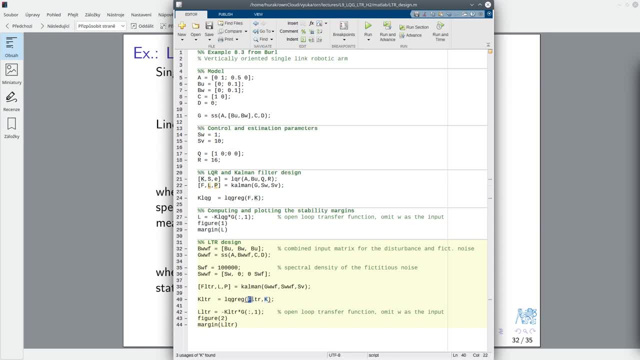 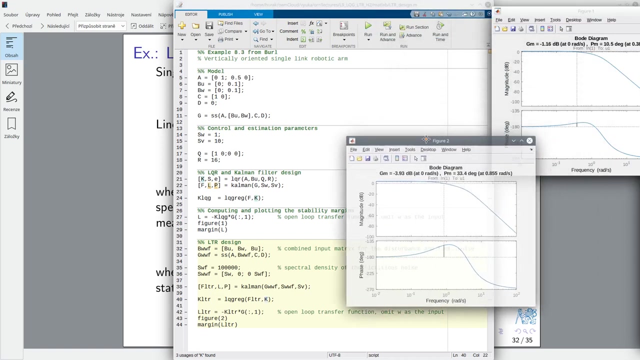 filter, with, with the, with the original state feedback, and that's it. and for this new LQG optimal output feedback controller we compute the open-loop transfer function and for this we also plot the open-loop frequency responses and compute the margin. so I time to run the code. so these are the 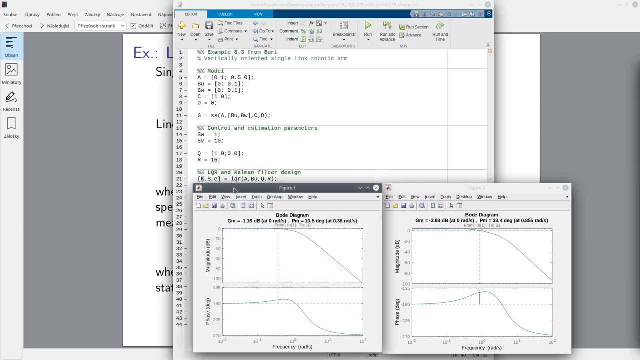 two frequency responses. so let's have a look at how it, how it works. so the first, uh, the first frequency responses, the ones on the left, are corresponding to the lqg design and we can see that the phase margin is some 10 degrees. again, margin is slightly more than than one decibel. 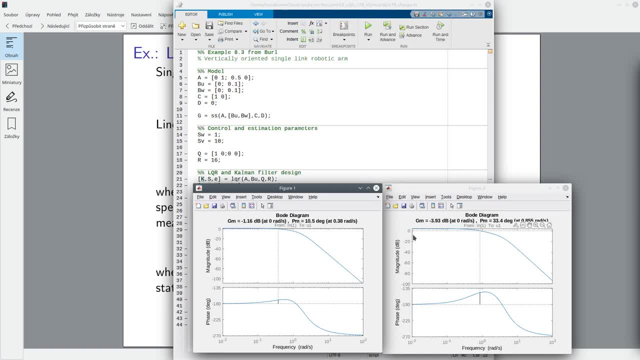 actually minus one decibel. so how, how is it with, uh, the, with the ltr design somewhat better right three or actually even four times better gain margin and similarly three times larger phase margin. so obviously somehow it's it works and it's it's really quite a usable procedure. so if you 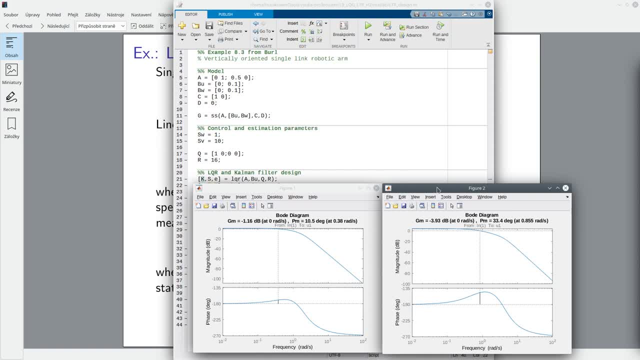 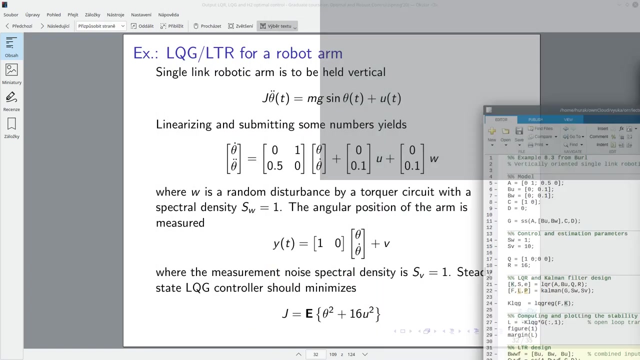 start using lqg stuff. it's a, not a. it's not a lost game. you can still keep using it and using these tricks, like ltr, you can improve the robustness, the insensitivity to, to modeling discrepancies somewhat. all right, that was it and let's move on again. 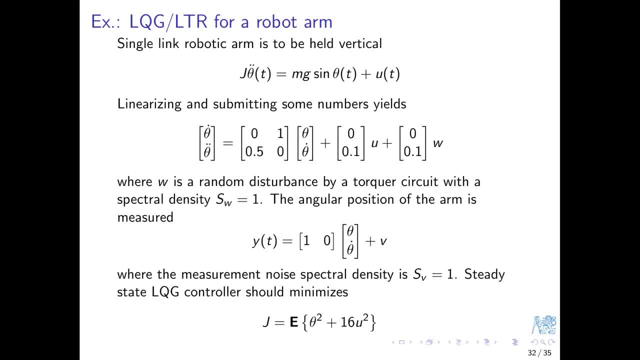 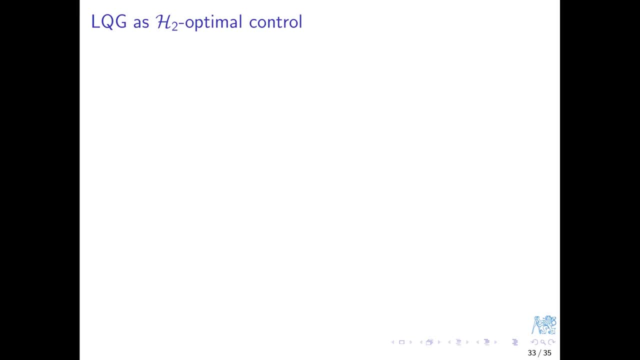 to the next one. so we are approaching the grand finale. what i would like to show you, finally, is that, similarly as we formulated the lqr design problem as an instance of the h2 system or minimization, we can also pose the lqg problem within the same h2 norm minimization framework. 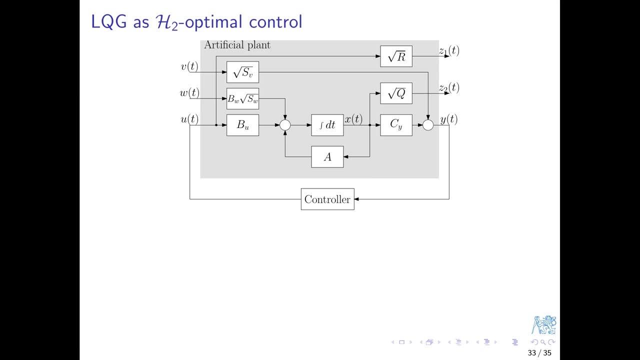 claim that the equivalent block diagram for H2NOR minimization is this: The gray block, the artificial plant, or actually more often called generalized plant in the community, now contains some new stuff with respect to the LQR situation. Let's go through all these systematically. First, we observe that we 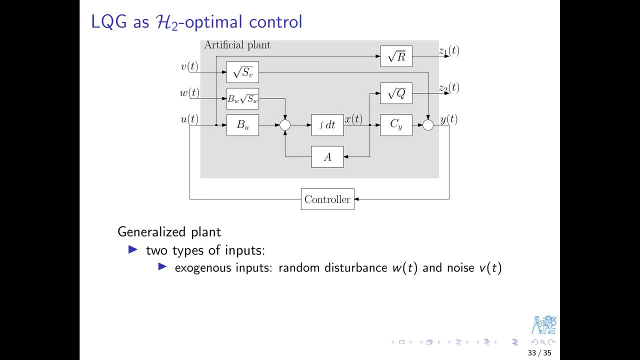 have again two groups of inputs. In the first group, also called exogenous inputs, we have the random disturbance W and the measurement noise V. What makes them valid members of this group is that none of these is under our control and they are only known to the extent that we know that they belong to some class of 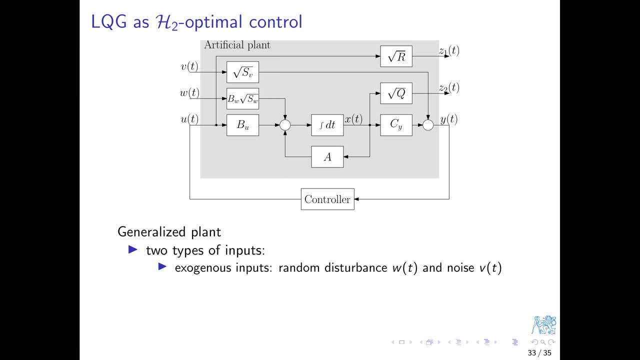 signals, Namely, in this case, they are white noises. If you now check the diagram carefully, you can see that they are white noises. If you now check the diagram carefully, you can see that these noises are actually assumed to be of unit spectral density because 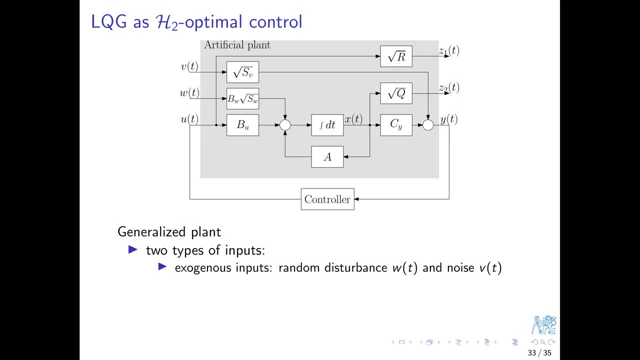 the generalized plant also already contains the blocks with SW and SV that scale the spectral density accordingly. Think about the reason for the square root there. The second group of input contains a single signal here, the control signal U. In fact, that's how the membership into this group is. 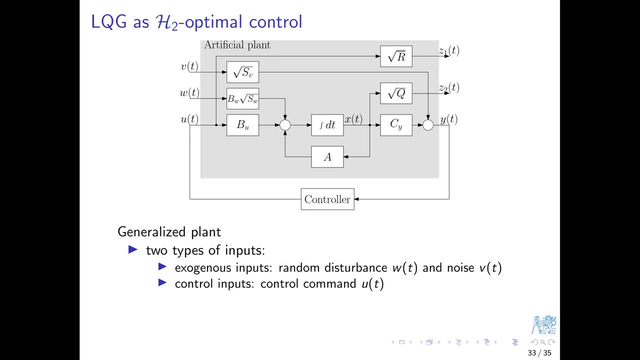 defined. These are simply the inputs to the system that are under our control. We can change these signals in real time arbitrarily in order to influence the response of the system. Obviously, membership in these two groups is exclusive. Either the signal belongs to one group or the other. 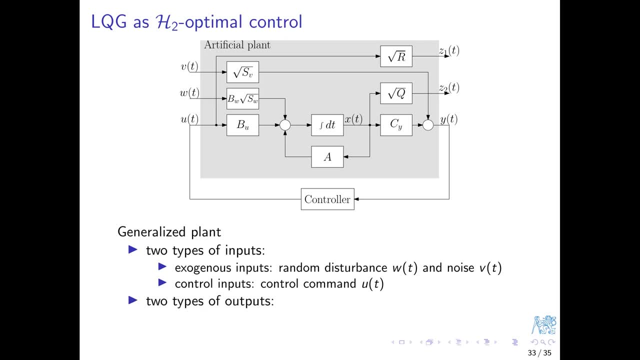 Good, Then we have two groups of outputs. The first group contains the signals Z1 and Z2 in our diagram. Generally we call these signals regulated outputs. This is to say that we want to make and keep these signals small. Small in some sense. 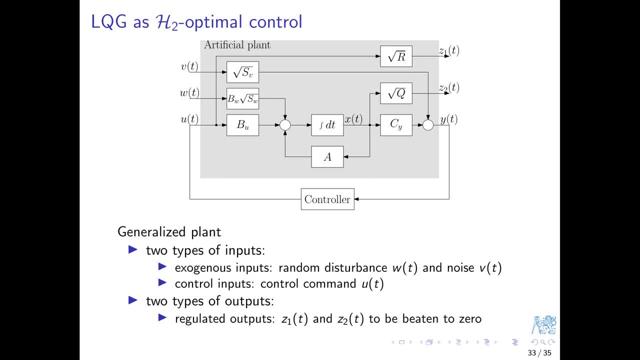 But this sense needs to be specified precisely, of course, But we already did it right. These signals should be kept small in terms of the mean square value. Finally, the second group of outputs: Y signal. In our case, membership into this group is defined simply by the fact that the given signal or variable is measured and fed to the controller for further processing. 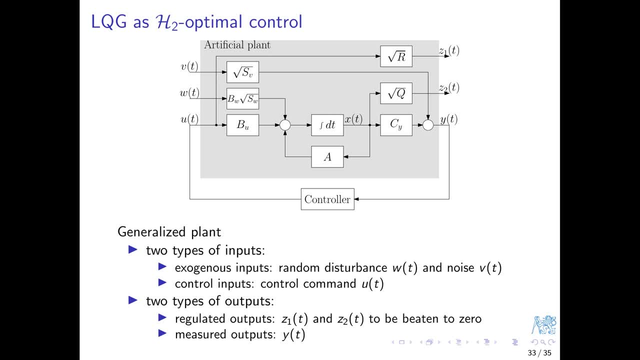 We call these simply measured outputs. Unlike in the case of the two input groups, here the membership is not exclusive. Obviously, we may want to keep some signals small, and yet we measure it and use it for feedback control. In our case, this did not happen. 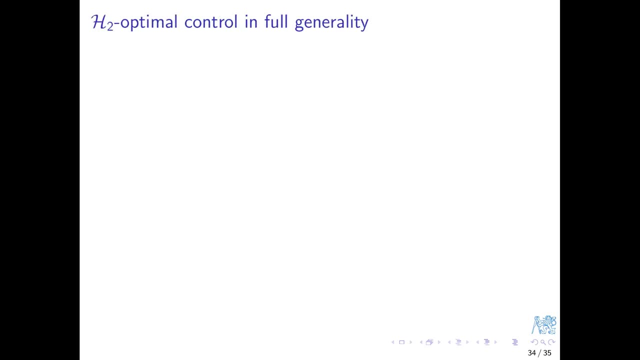 But generally it could be the case. This brings me to generalization of the proposed control design scheme. The task for the designer is to formulate, to build the generalized plant, say P, with two groups of inputs and two groups of outputs, with the roles that we have just defined. 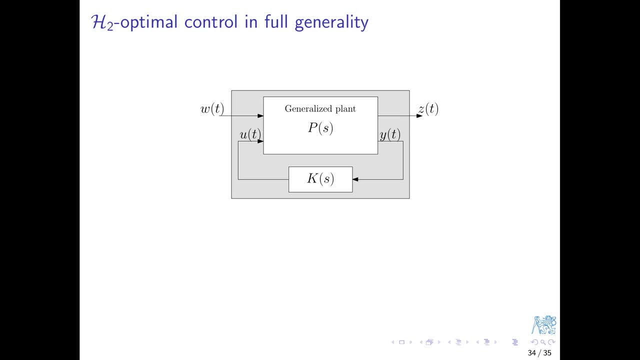 What's inside the P block is up to the designer. It could be exact. It could be exactly what we had in the case of LQR and LQG designs, But it could also contain some modifications and augmentations on top of these. 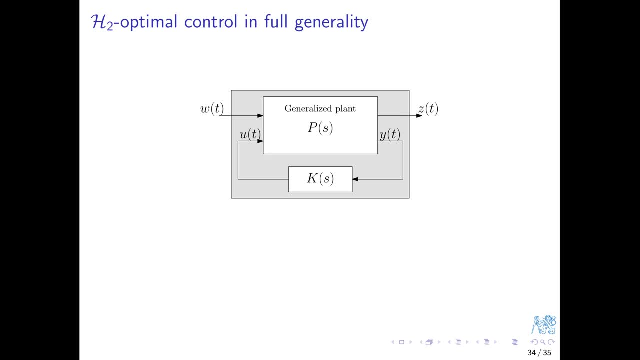 For example, some first or second order filters could be added to the exogenous input signal paths to account for the fact that the inputs are not exactly white noises but, rather more realistically, something called colored noises with frequency-limited spectrum. The crucial thing. 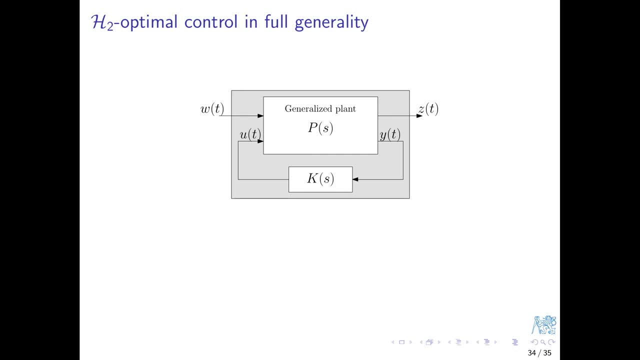 The crucial point is that the inputs are not exactly white noises but rather, more realistically, something called colored noises with frequency-limited spectrum. The crucial property of this generalized plant is, however, that if the regulated outputs are pushed towards zero in some sense that we have just discussed- 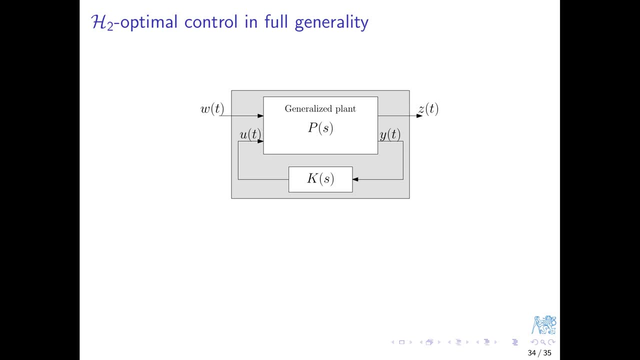 the control specifications are satisfied, You see what I mean. You really need to formulate this P system such that, if some- possibly even artificial- signals are pushed to zero, you get from your physical control system exactly what you wanted. Once the generalized plant is specified, the role of the designer has been essentially fulfilled. 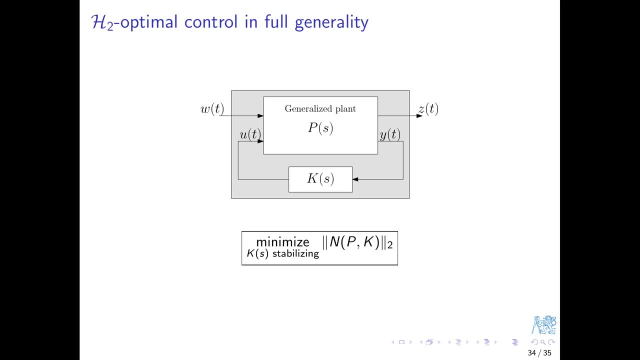 because what remains is a purely computational task of minimizing the norm with some stabilizing controller. The N function inside the norm stands for this special feedback interconnection of the generalized plant and the controller. Special in that only a subset of inputs and a subset of outputs are used for feedback control. 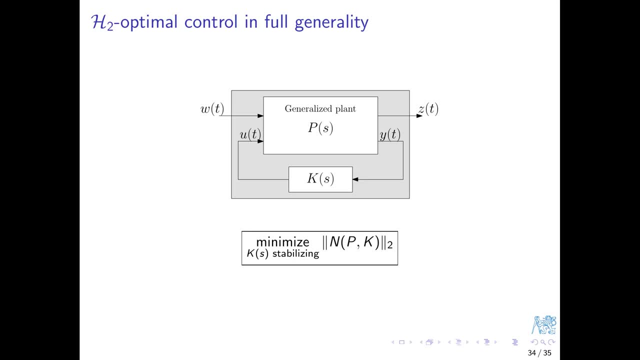 We will later discuss this a little bit more and we will name it, this whole feedback interconnection, as a so-called linear fractional transformation. Well, now, this well-defined problem has been rigorously studied and numerous numerical solvers exist. Our plan in this course is not to go into the mathematical details. 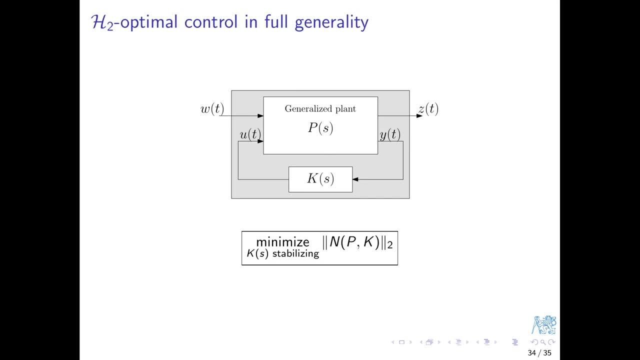 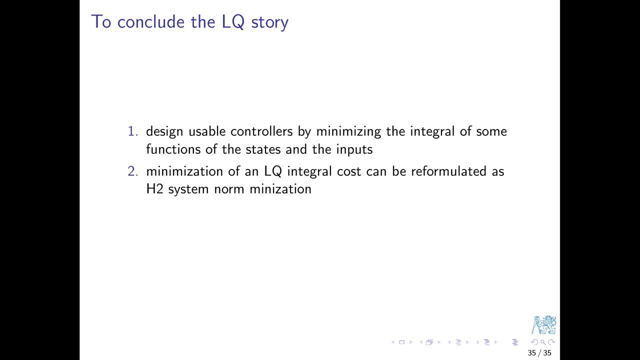 Instead, we find ourselves more in the position of users of such computational tools, And this is essentially the end of our LQ story. We've not only learned to formulate control design problems in the optimization framework, in which the cost function is an integral of some